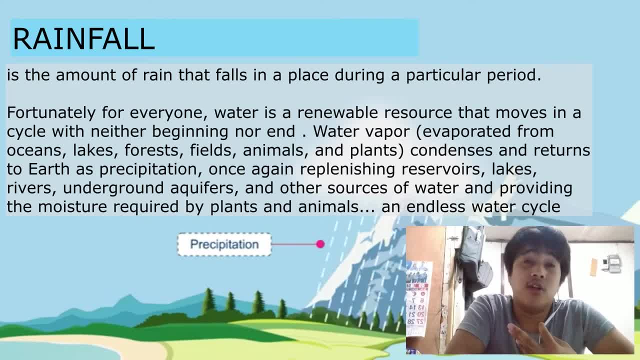 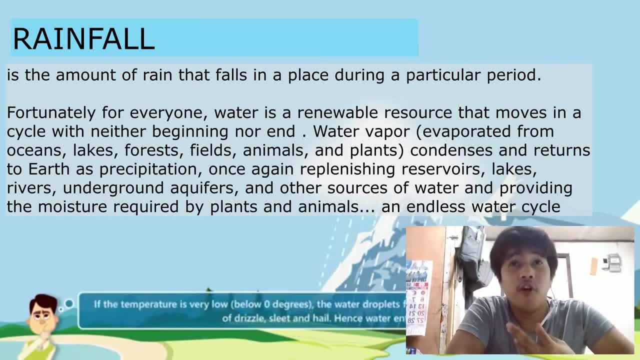 And, according to the dictionary, the amount of rain that falls in a place during a particular period is called rainfall. Fortunately for everyone, water is a renewable source that moves in a cycle with neither beginning nor end. Water vapor, evaporated from the ocean, lakes, forests, fields, animals and plants, condenses and returns to earth as precipitation. 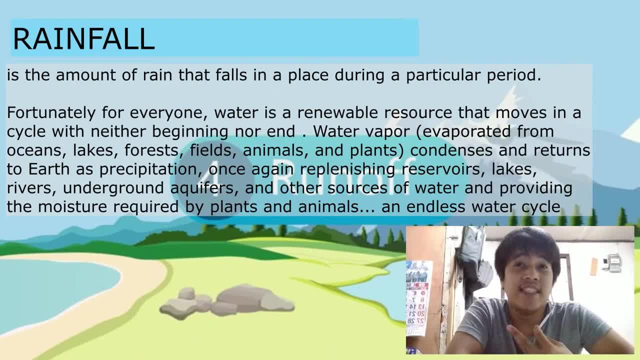 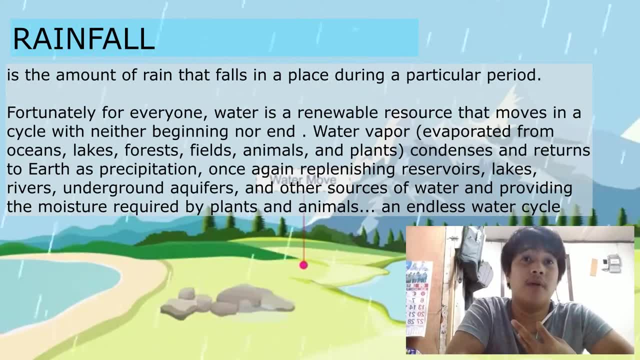 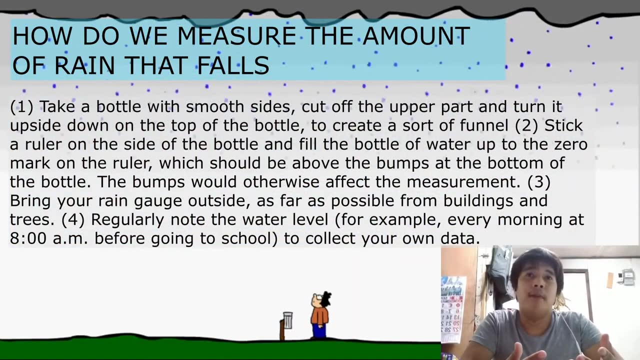 Once again replenish the reservoir, lakes, rivers, underground aquifers and other sources of water And produce water Providing the moisture required by plants and animals. An endless water cycle. How do we measure the amount of rain that falls? 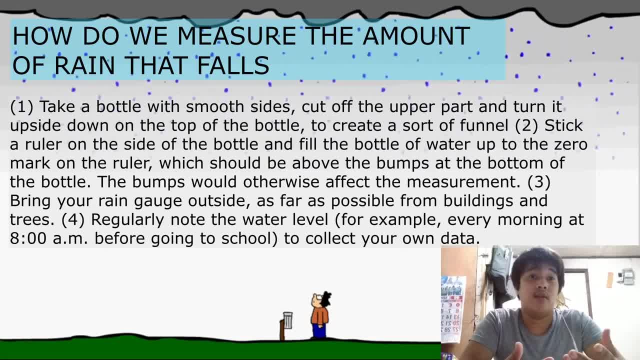 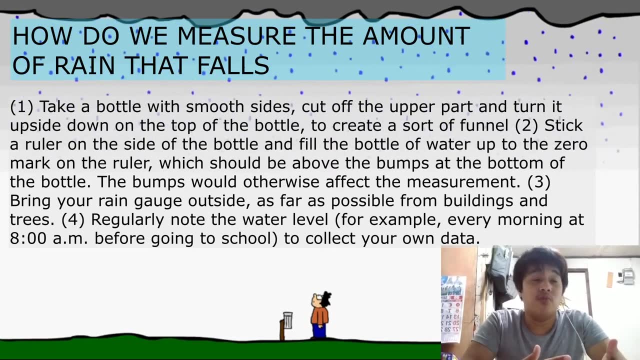 Actually, there's a lot of methods or ways or equipment to measure the amount of rain that falls in a certain area, But let me teach you a way, a DIY or do it yourself method, which you can do at your home for experiment. 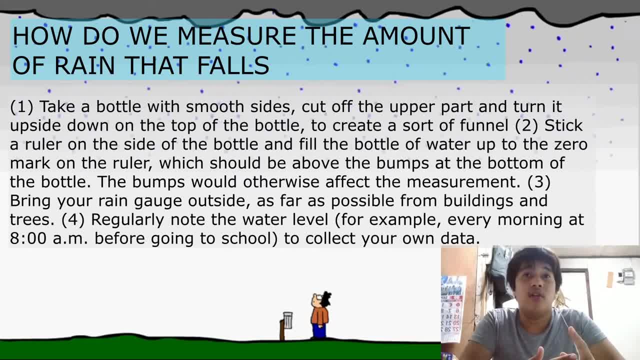 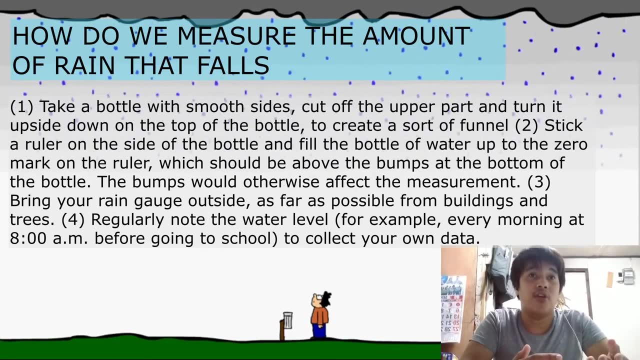 So, first of that, take a bottle with a smooth side, cut off the upper part and turn it upside down on the top of the bottle to create a sort of funnel. Stick a ruler on the side of the bottle and fill the bottle of water up to the zero mark on the ruler, which should be above the bumps of the bottom of the bottle. 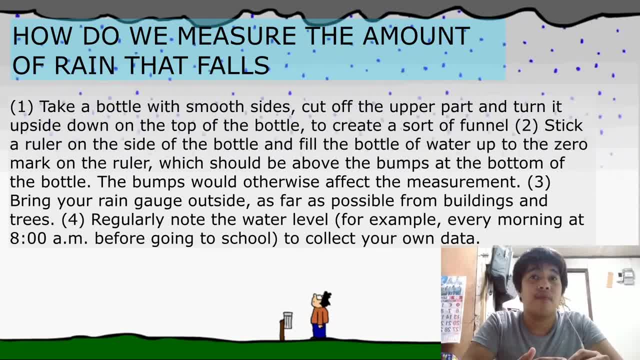 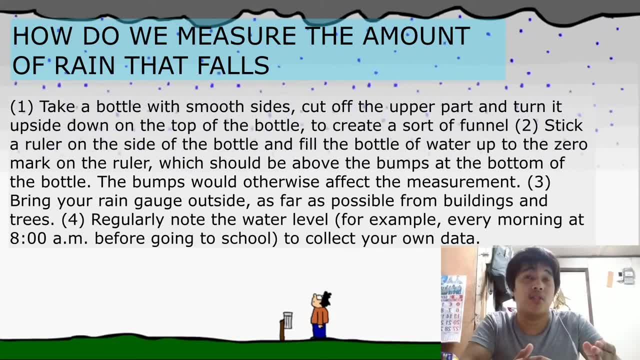 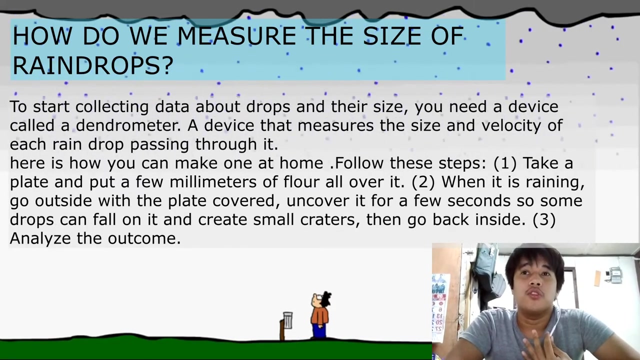 The bumps would otherwise affect the measurement. The, The, The, The, The, The, The Is The, See the. The oil is less dense, so it will go up to avoid the water to evaporate. So how do we measure the size of the raindrops? So actually there's a device, which called a Tentrometer, that measures the size and velocity. 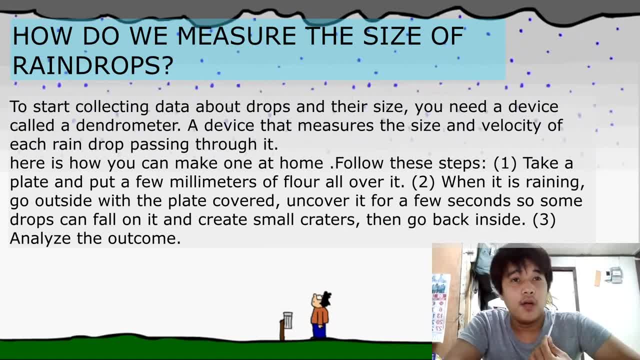 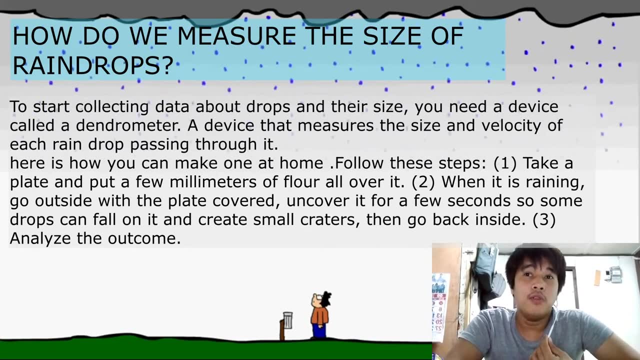 of each raindrop passing through it. But in this video I will teach you a DIY or DIY method which you can do at home and make this experiment. So first is take a plate and put a few millimeters of flour all over it. Then, when it is raining, go outside with plate covered and cover it for few seconds. so some. 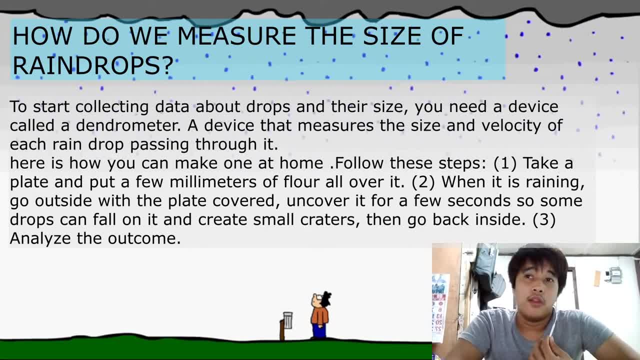 drops can fall on it and create small craters. Then go back inside and analyze data. You will notice that the drops do not all have the same sizes. Some are very small and some are very large. The creators are bigger than the drops because the water slightly spreads all over the plate. 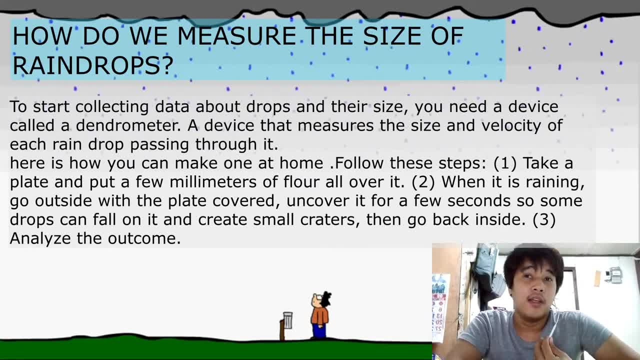 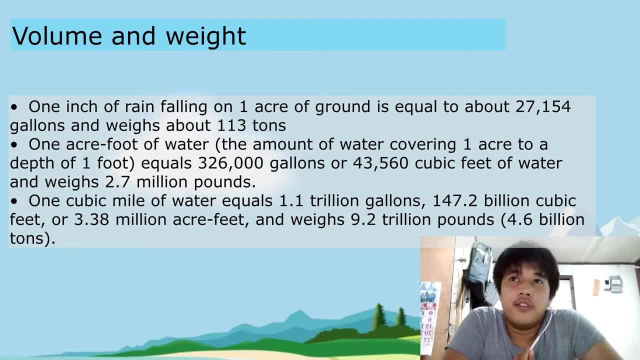 But they still enable you to directly visualize the great variety of drop sizes, even during a short time. Here is the water equivalent of rainfall For the volume of weight: 1 inch of rain falling and 1 acre of ground is equal to 27,154 gallons. 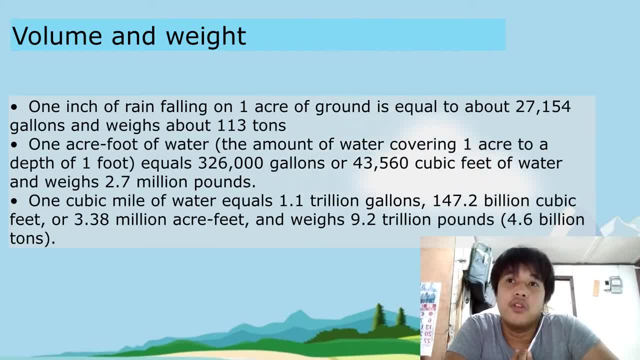 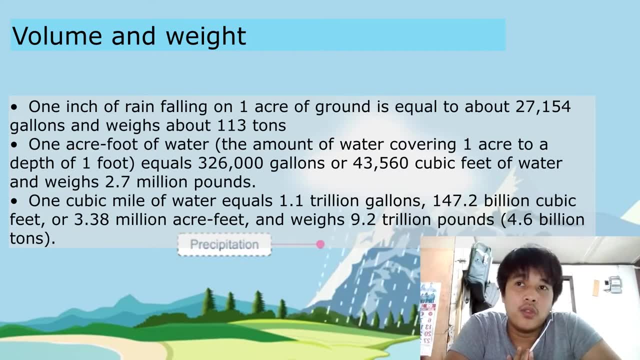 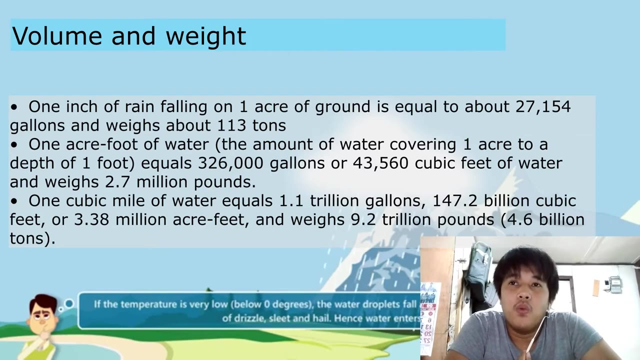 and weighs about 113 tons. One acre foot of water. the amount of water covering one acre to a depth of one foot equals to 326,000 gallons or 43,500 tons. So that's it, Thank you. The figure is equal to 163,560 cubic feet of water and weighs 2.7 million pounds. 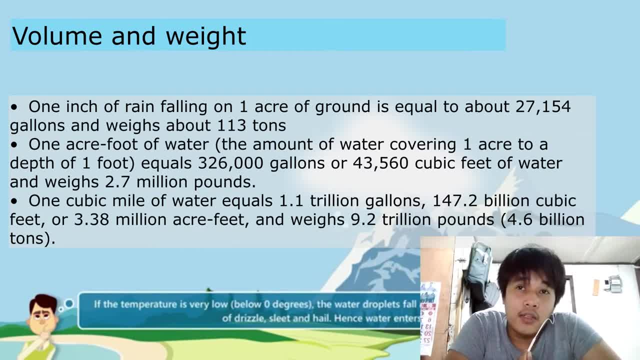 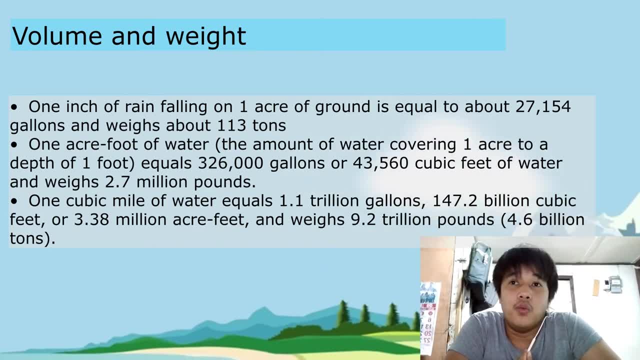 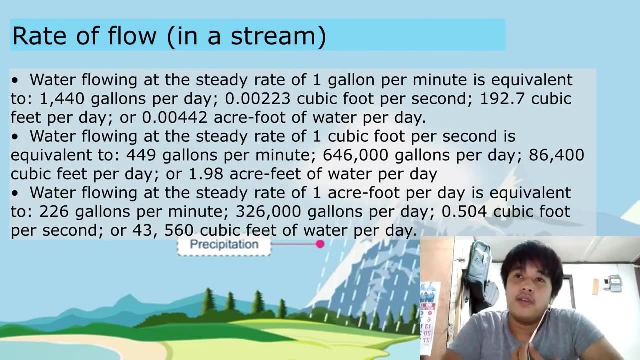 One cubic mile of water equals 1.1 trillion gallons or 147.2 billion cubic feet, or 3.38 million acre feet, and weighs 9.2 trillion pounds, or 4.6 billion tons, For the rate flow in stream. 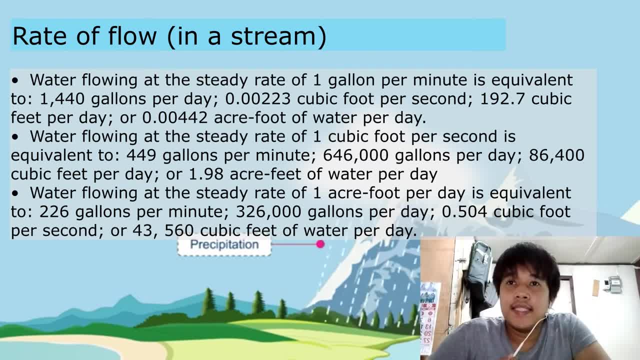 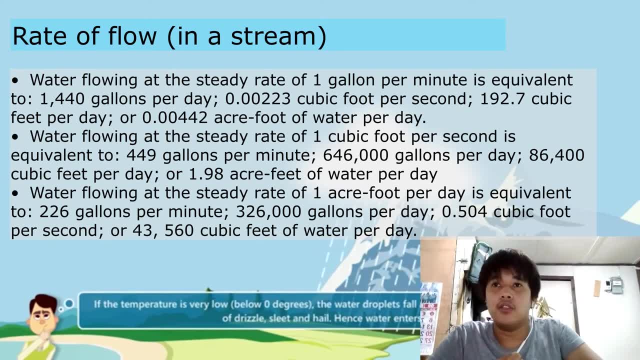 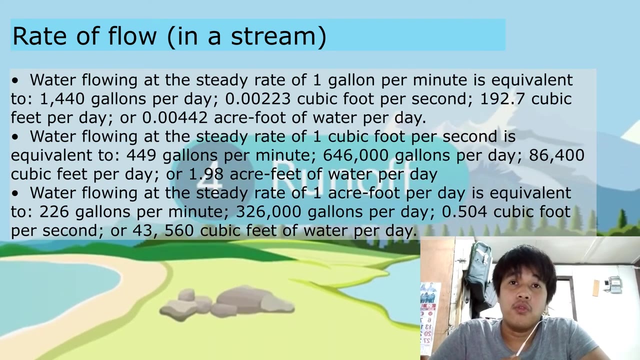 In stream Water flowing at a steady rate or 1 gallon per million is equivalent to 1,440 gallons per day, or 0.00223 cubic feet per day, or 0.0047 acre-foot of water per day.